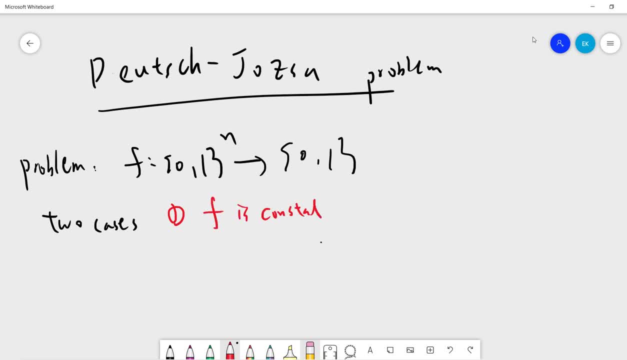 the first case is f is constant, so that means uh, for all x belongs to zero, one to the n. f of x is either zero or one. okay, and the second statement, the second possibilities, is that. so the second possibility is that the F is balanced, so this means half of. 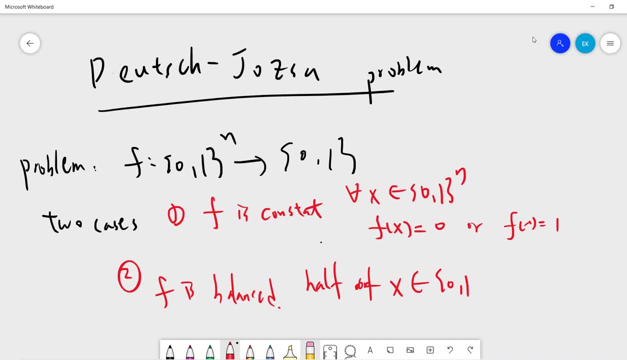 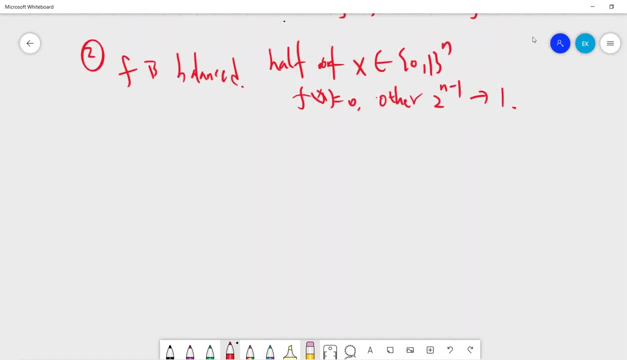 X, half of X in the zero. one of n will give you zero and and the other other will. other two to a minus one number will give you one. okay, so this is the two case of F. so the goal is to determine, determine which F now which? 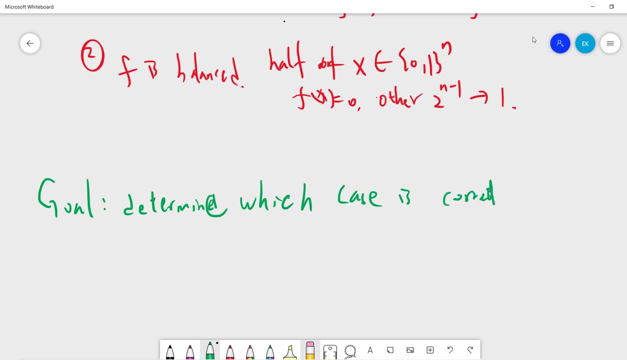 cases is correct. so we need to, we need to design the algorithm. so for the classical one, so the classical one, you need to first choose one, choose one of them, and if you get one, and if you choose another X, then you get zero. then you know that, oh, it must be balanced. so the optimal case for the 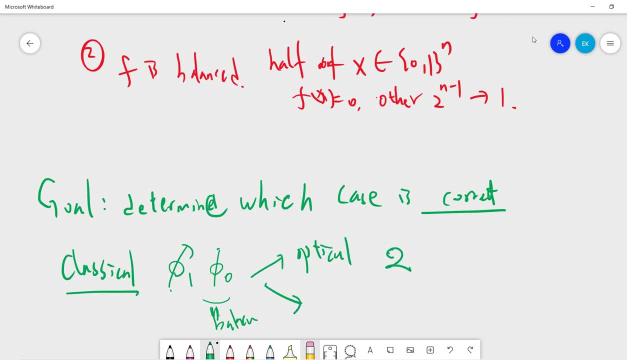 classical is you need to compute twice and, and the worst case is you, you, you, you get zero, zero, zero, zero, zero, and on, and you, you take two to a minus one times and finally you get the rest. if it is still zero, then you know it's constant, if it's one. 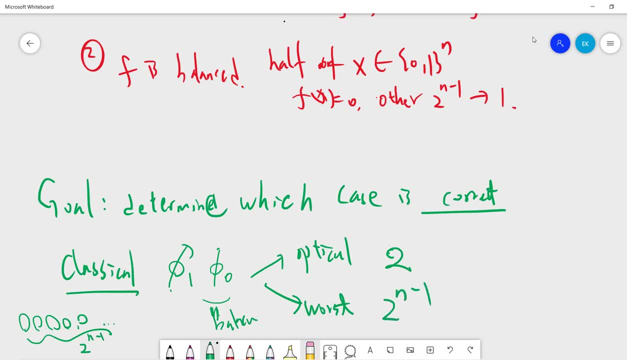 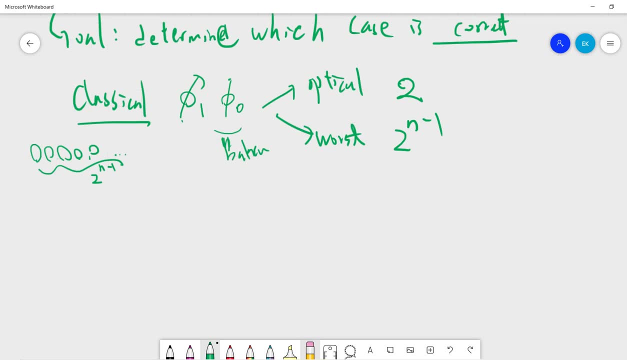 then you know it's balanced. so the worst case is two to a minus one. okay, so this is the classical one. so if its very large, then basically you only exponential type. that is for exponential type. okay, so this is our quantum algorithm. basically you have some zero. 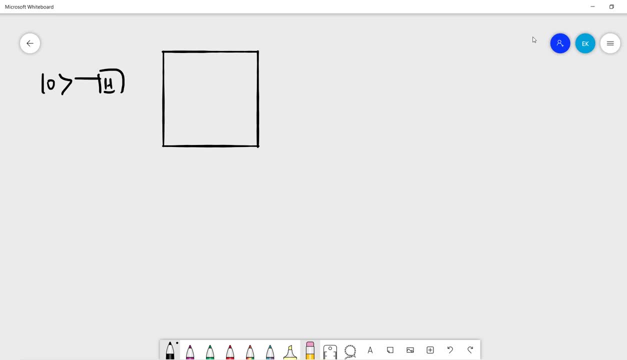 you go to the hardware case and then you, By the way, this is 0,, 10,, 7,, so 0,, 10, 7, and then this is a hard mark gate, okay, and also 1, and then you go to hard mark gate and go into, and then after that you go to. 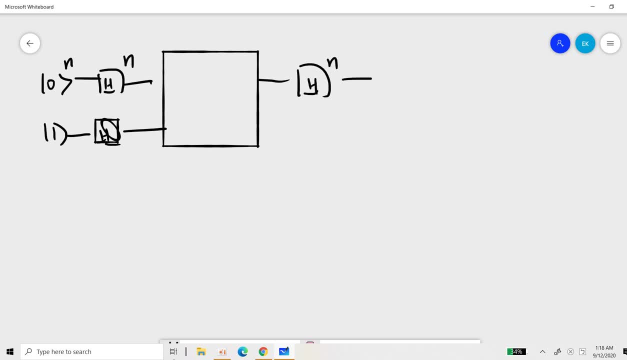 another hard mark gate, basically hard mark 10,, 7, and then you go to measure this, measure the first, 1, and then this is just passing. So this is just n theta, so this is doesn't, does not have important meaning, okay. 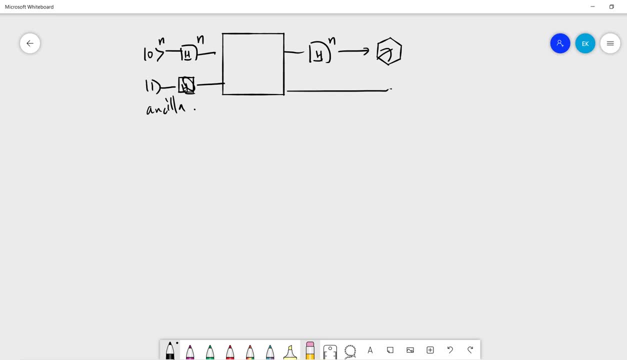 So before proving it, we first need to know something really important. So if you have tensor n and then you get hard mark n, then you will have this basically- you need to remember this- and you will get 2 to n and basically, since x is from 0 to 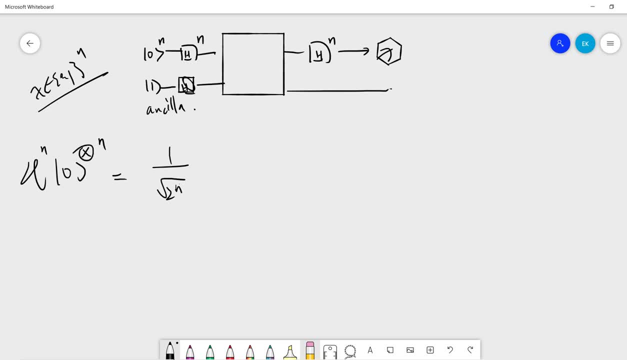 n so we can map the quantum state, So we can just use this notation from 0 to 2 to n. okay, minus 1, okay. so this is things you need to remember. and the last thing is that if you add on something called x, then 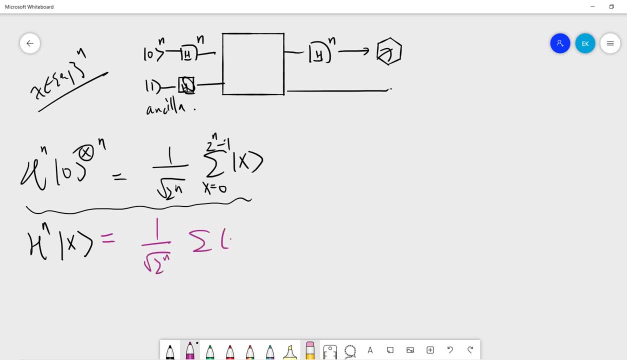 you will have 1 over square this 1, and minus x, dot y and the y is also from 0 to 2 to n minus 1.. And this is the bitwise product. Okay, So, bitwise product, I mean just, you can write x into vector x1,, x2,, xn and the y. 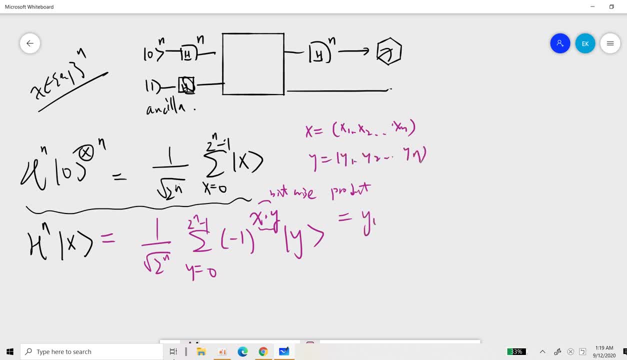 just y1,, y2, yn, and this product just y1, x1,, direct sum x2, oh, so this is the. let me see, this is should be the should be, should be what? Oh? 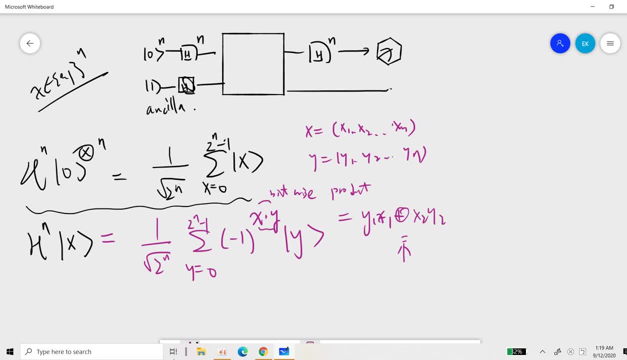 Oh, it's just so. this is just bitwise product. so so if this, yeah, 2, 0, 0, you get 0, and 1, 0, you get 0, and 1, 1,, you get 1,, and then you just this. so this is just like a parity. 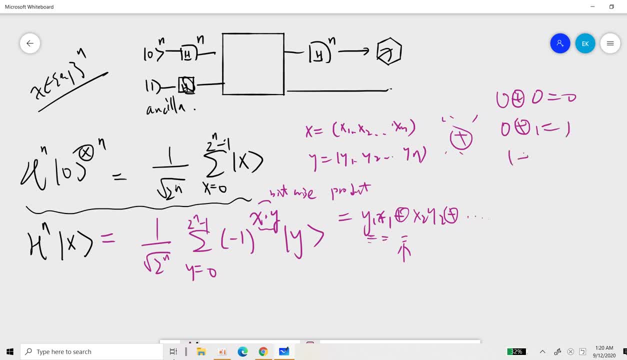 so it's 0, add 0, it's 0, and 0, add 1, it's 1,. 1, add 1, it's 1, and 1, add 1, it's 0.. 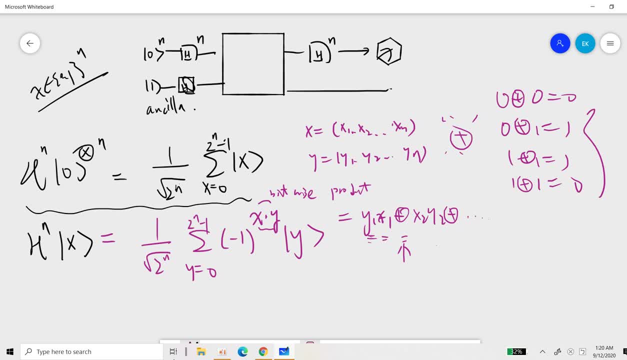 Okay. So basically, you just So each of x should be 0. Okay. So if you get 0, 1, then you can compute this and compute this, compute this, Okay. So this is the thing you have to remember. 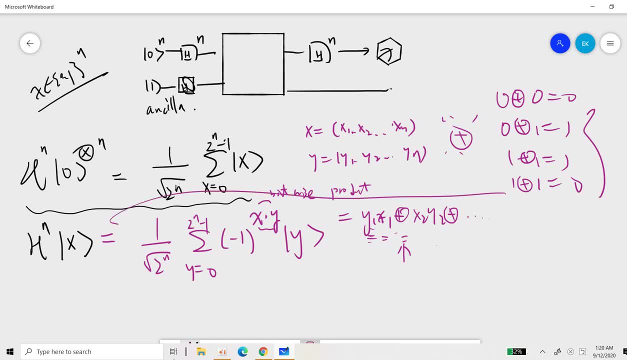 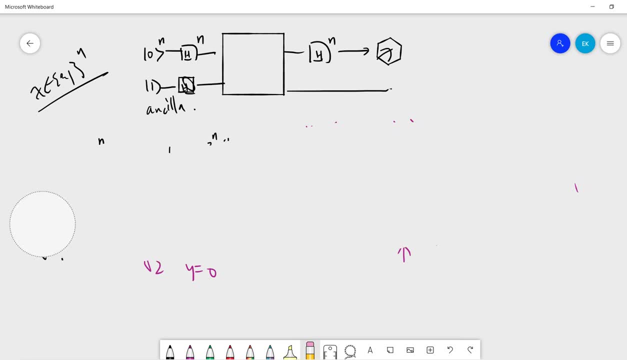 Okay, So once you have remembered this, then we can start to do the, the algorithms analysis and see why this is correct. I mean this is very amazing that I mean when the first time I saw these algorithms, because I mean it's very, very 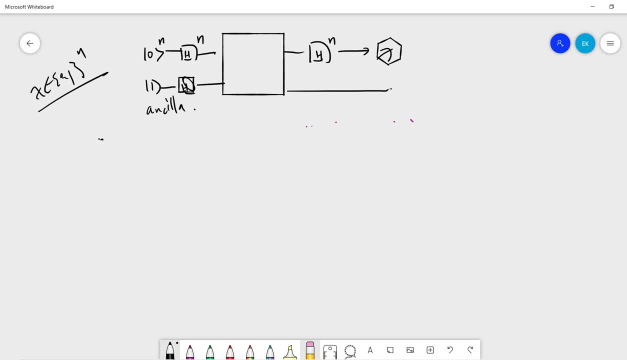 Yeah, Yeah, Very strange that this is something which all can work. Okay, So the list state this state, this state 5 is just the Hadamard gates of 0, so you get this one minus. I'm sorry what I'm writing it for. 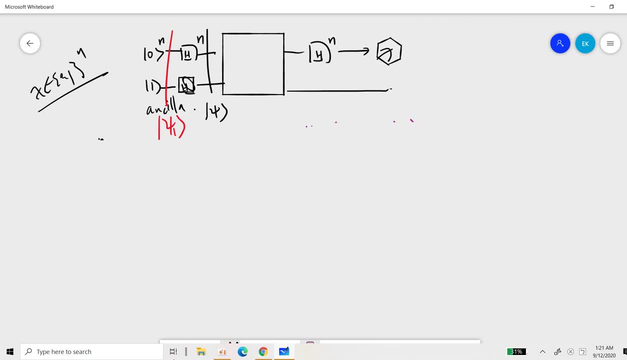 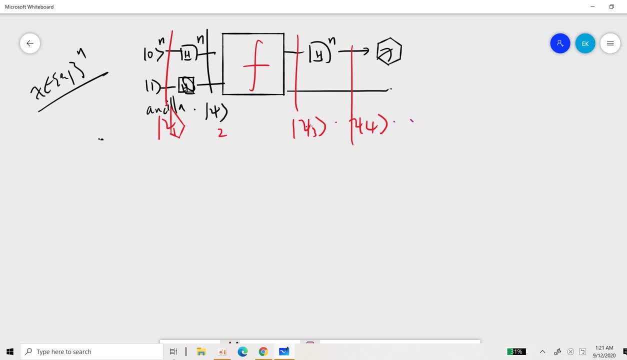 5, 4,. basically the function f is here, okay. so 5, 1 is just this, okay, and 5, 2 is just: you take Hallmark gates of the 0, n and the Hallmark gate of 1, and you tensor product. so this will give you 2 to the n plus 1, x, x from 0 to n minus 1, and 1, oh sorry, this is 0 minus 1, okay. 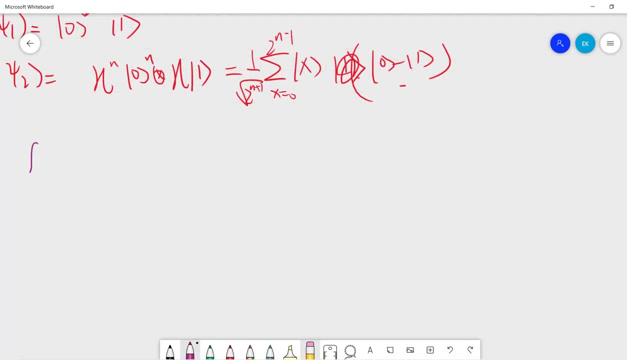 and then you finally take f. okay, so the f on the x, y will give you the x and the y, bitwise product x. so this is the quantum circuit, the quantum circuit you need to build. okay, so let's assume that you already know this. so you take this, then you will get this. 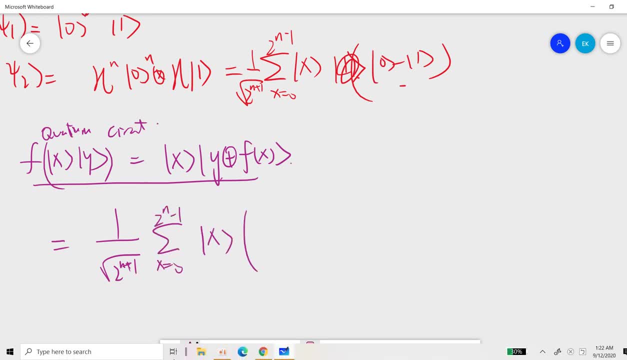 so it's very happy that you don't need up to now, we don't need- a quantum Fourier transform. okay, so you will have this. let me see you will have 6x. so you will have what f of X, because P, Y 0 is. 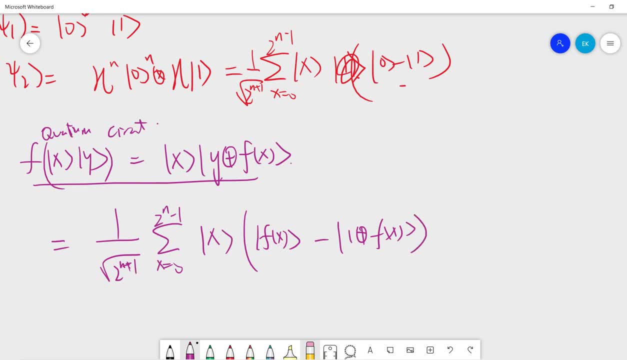 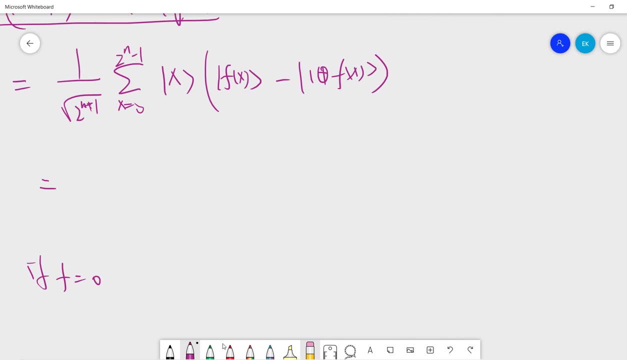 0 and P Y, f of X. okay, okay. so the important thing is that if f of 0, f of X is 0, then let's turn 0 minus 1, and if f is 1, then its one minus 0, so you can. 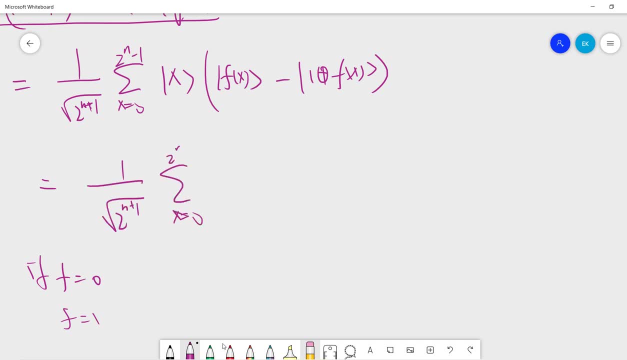 write this list minus X. so this is the key importance step. here you can write s this: 0 minus 1, okay, okay, so from here, then we can, so we add on here, so now we have our我就 need five, three, so if five four. another point: five, four step, so if five four. 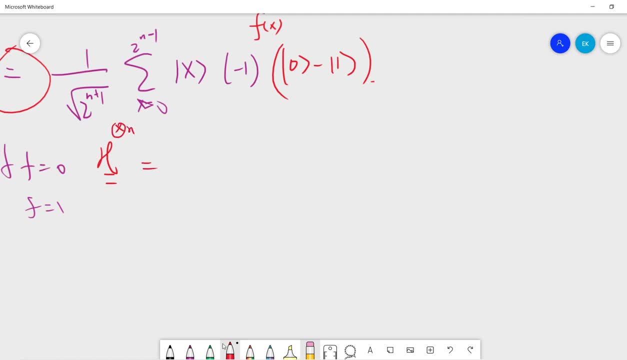 we just add hard market at the first side at this part. okay, so I will get this: 2 to the n plus 1 and 1 over 2 to the n, and still x equals 0 to n minus 1, and then pick on y and minus x dot y and then there is a y, so y from 0 to 2 to n minus 1. 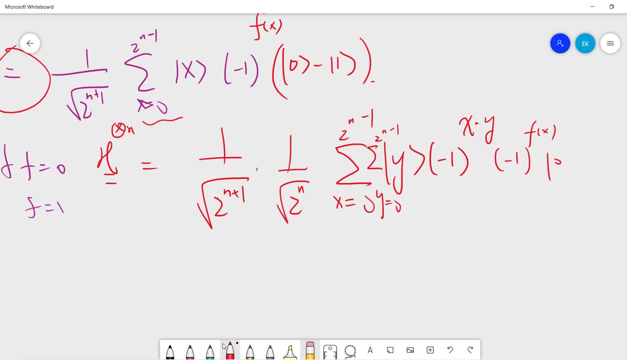 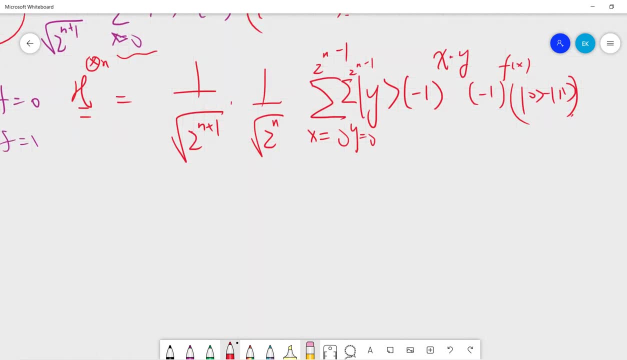 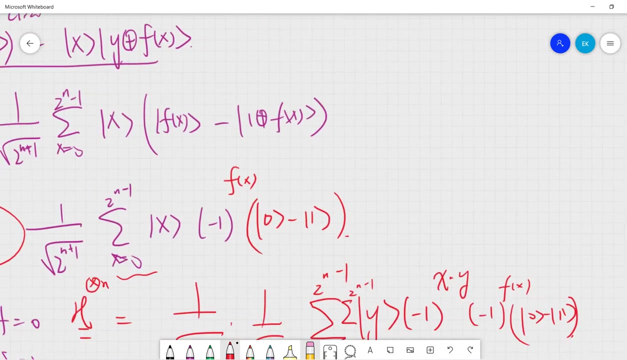 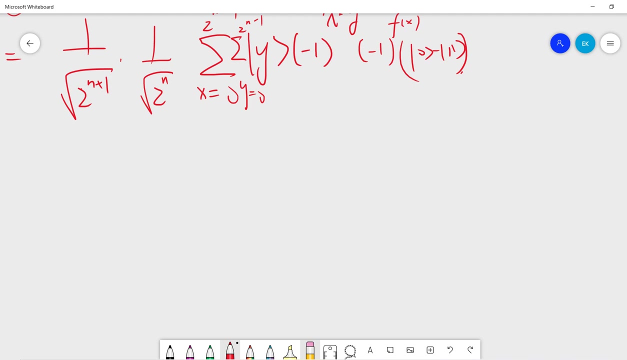 and then minus f of x, and then 0 and minus 1. okay so, and okay so, let me killing the result. okay, so, basically, this is 0 for 1 and we only first measure first. ok, so we didn't care about it, so we can just, since it's tensor product, so we can. 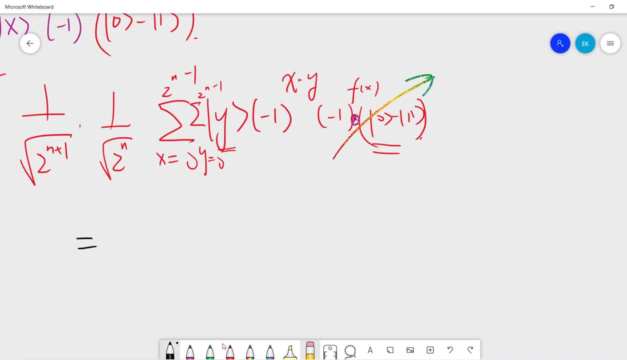 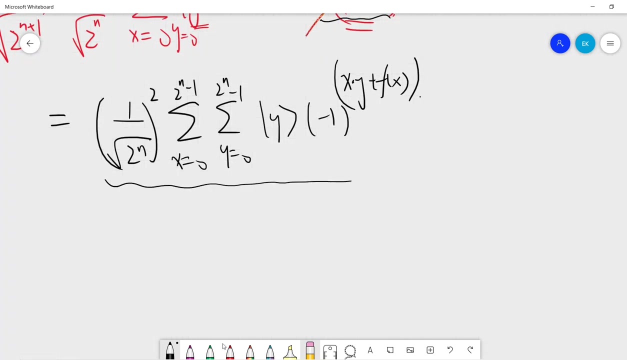 just ignore this, so we will have the final state: look like this square, since I already take one over square, root, two to cancel it, to pull these things out. so this is the final result. okay, so basically is y minus X bit, Y plus f of X, nice, nice, so it's one over two to n: X, Y and Valet minus. 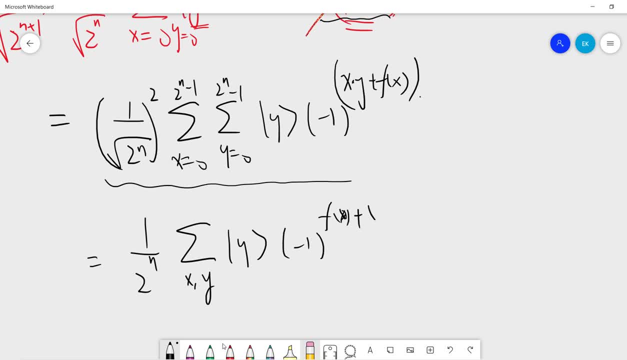 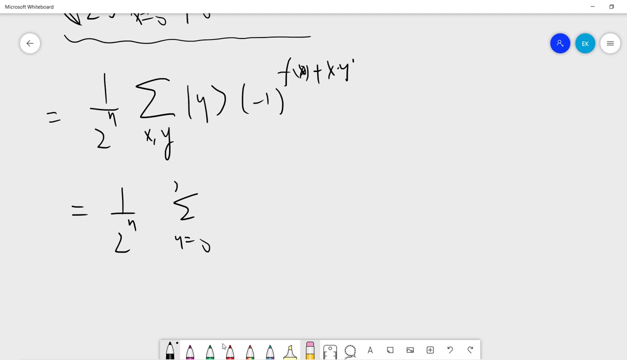 f of X plus X dot Y. okay, okay, so, okay, so I didn't write it down. 1 over 2 to the n y, from 0 to minus 1, x from 0 to the minus 1, and minus 1 f of x. 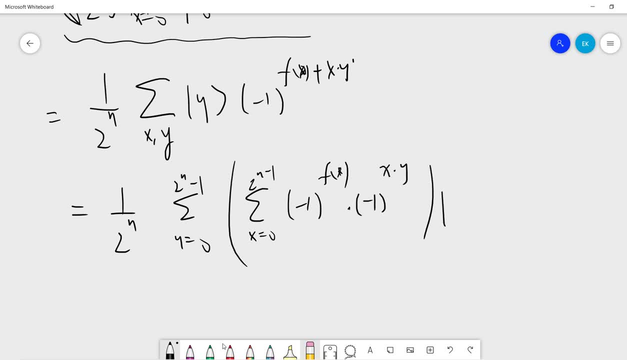 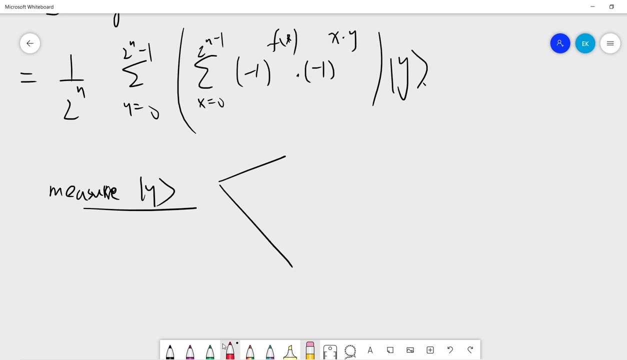 minus 1 x bit yy and the y. okay, then finally, finally, I just measure, I just measure y, okay, so there are many possibilities. so the first possibility is that in the first case, if f is constant, that means minus f of x is just so. so since if I take okay, so so let me write it down. so the 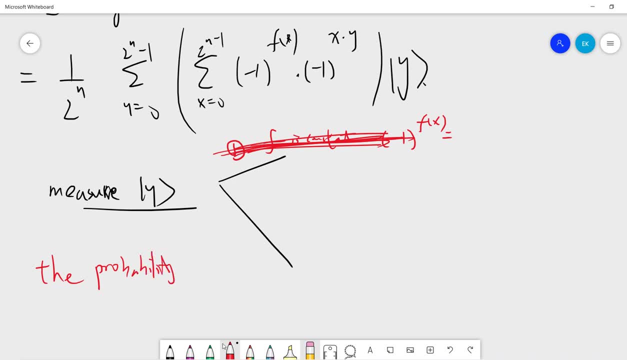 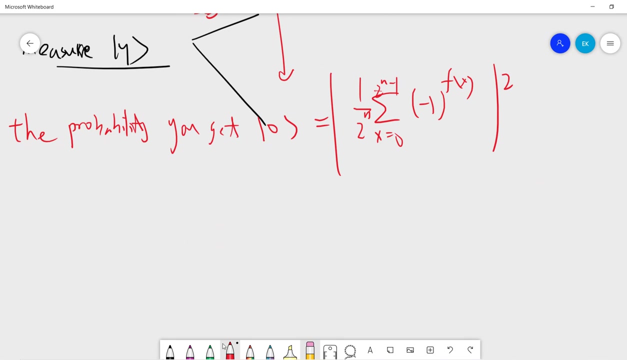 probabilities. the probability is you get 0 is just square root of 1, y 0. so 1 is 0, you just get 0. so this is just this okay. so the probability you get zero is this. so if f is in the first case, in the first case, if 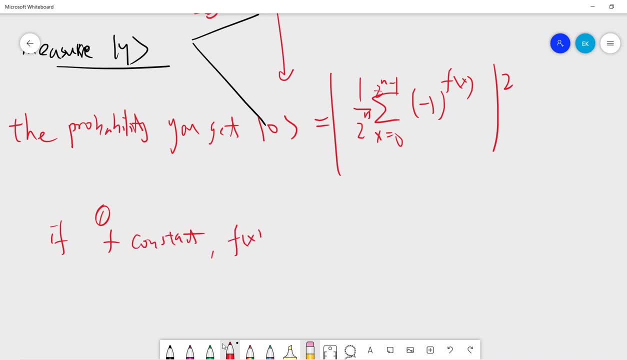 f is constant, then f of x is just constant, so this term is just minus one. if f of x is zero, and then you get the one plus one plus one plus one, and then this will get the p of zero is one. so you always get, you always get. 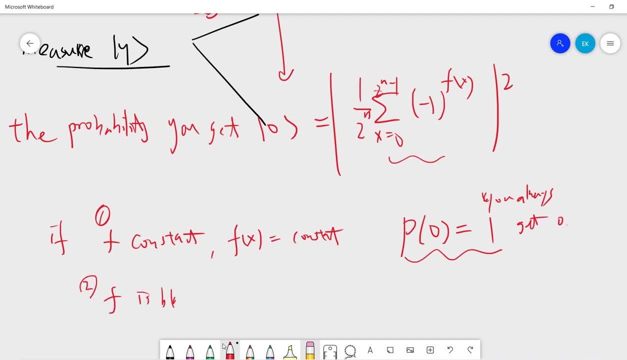 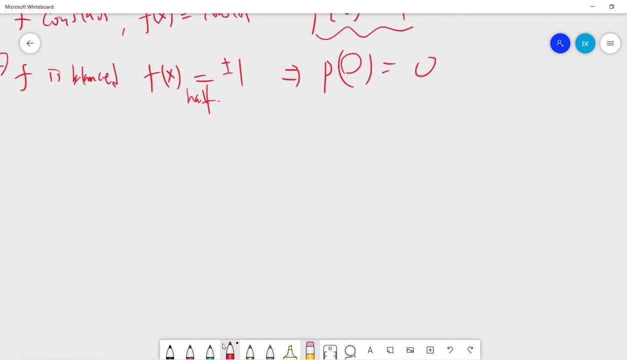 zero, okay. and the second: if s is balanced, uh, then f of x is uh, plus one plus or minus one and half half, so this term will be zero. so you'll get p of zero, which is zero, okay. so who's telling you that you can just. you can just measure one time, you can just measure. 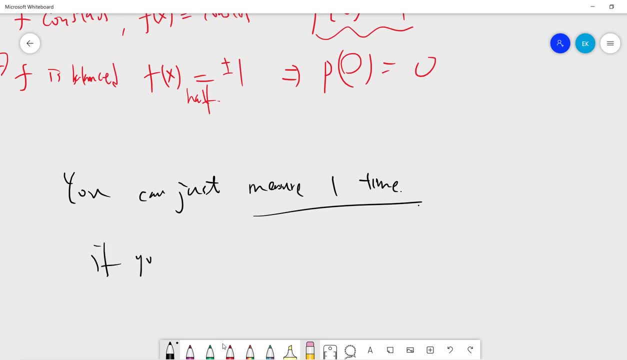 one time. if you get zero, then you know that basically is constant, and if you get one, basically it's balanced. so you only need all one time. okay, and deterministic. so compared to the, the classical one. so for the classical one you need uh, uh, average, you need uh. 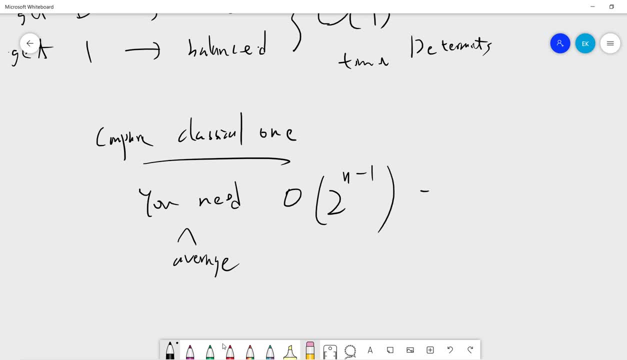 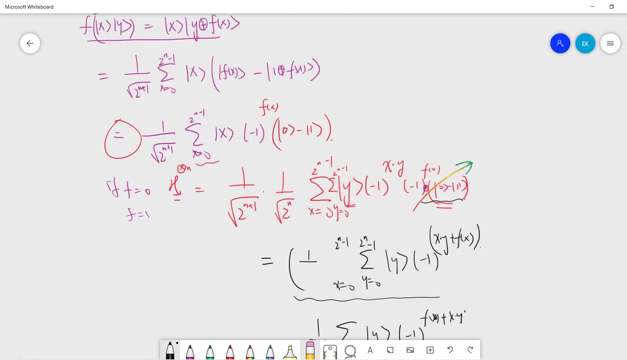 all to a two and uh minus one uh time. okay, so basically, uh, from this uh very stupid example that you can see the quantum, quantum algorithms, uh, in definitely have some. uh may have some uh much difficult, uh much a powerful uh uh complexity or the behavior than the classical. 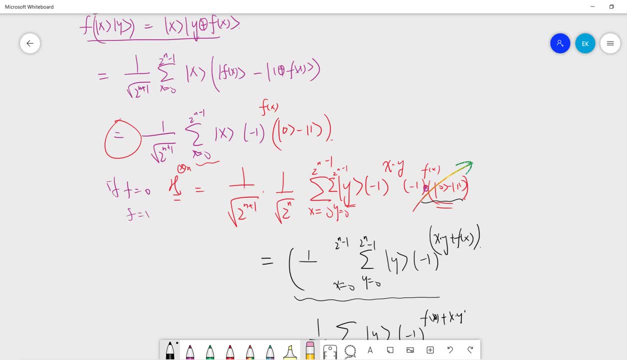 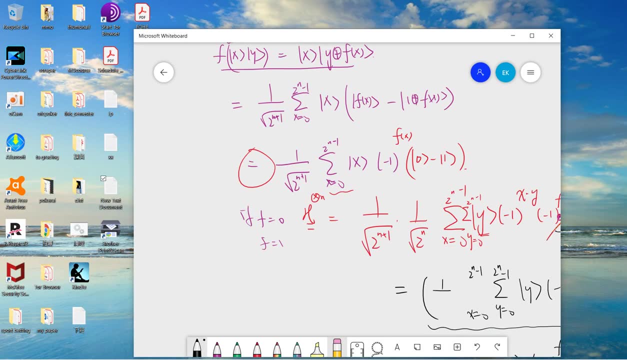 computer. okay, so this is the first corner algorithms i want to provide, which is interesting, and i will provide some interesting quality algorithm in the future. okay, so thank you and be sure to subscribe to my channel. thanks,